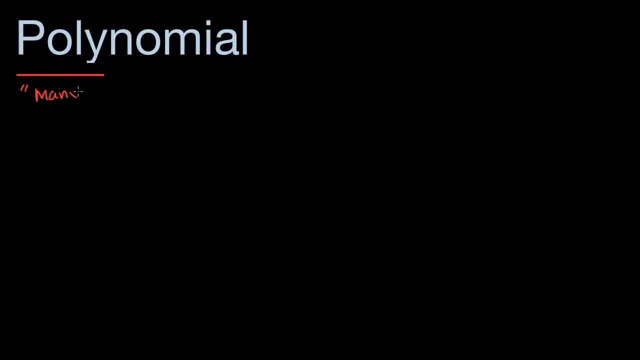 we have poly. This comes from Greek for many, and you see poly a lot in the English language referring to the notion of many of something. So in this case it's many nomials, and nomial comes from Latin, from the Latin nomen, for name. 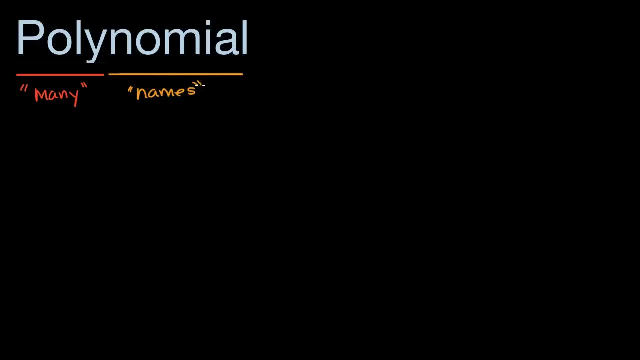 So you could view this as many names, but in a mathematical context it's really referring to many terms and we're gonna talk in a little bit about what a term really is. But to get a tangible sense of what are polynomials and what are not polynomials, 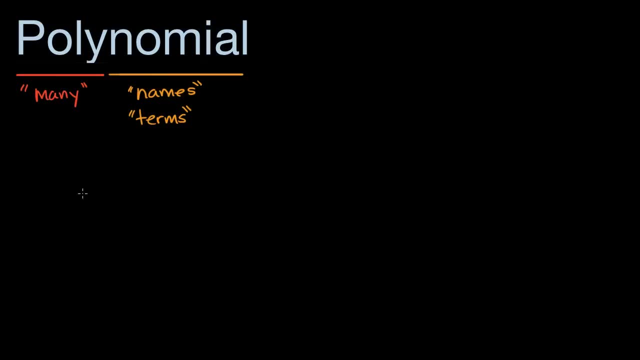 let me give you some examples and then we could write some maybe more formal rules for them. So an example of a polynomial could be: 10x to the 3rd, That's the 7th power minus 9x squared plus 15x to the 3rd plus nine. 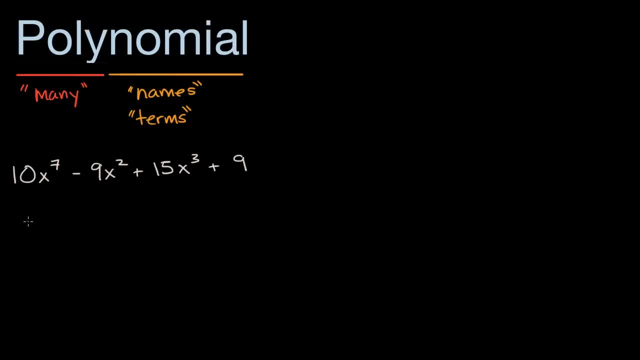 This is a polynomial. Another example of a polynomial: 9a squared minus five. Even if I just have one number, even if I were to just write the number six, that can officially be considered a polynomial. If I were to write 7x squared minus three. 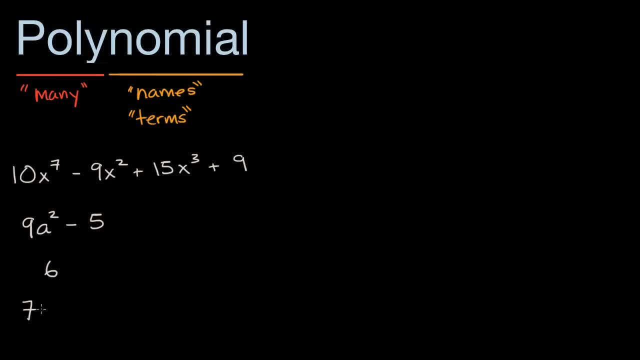 that's a polynomial. Let me do it in another variable: Seven y squared minus three, y plus pi, That too would be a polynomial. So these are examples of polynomials. What are examples of things that are not polynomials? Well, if I were to replace the 7th power right over here, 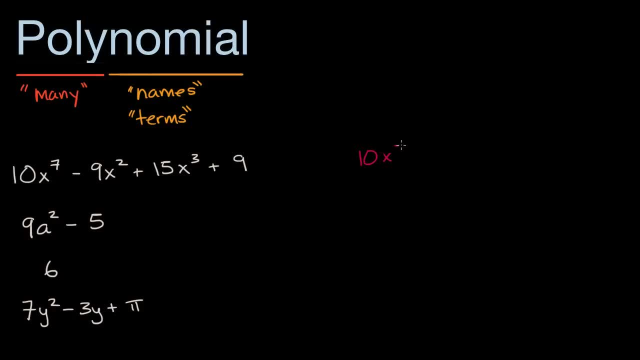 with the negative 7th power. so if I were to write 10x to the negative 7th power minus 9x, squared plus 15x to the 3rd power plus nine, this would not be a polynomial. So I think you might be sensing a rule here. 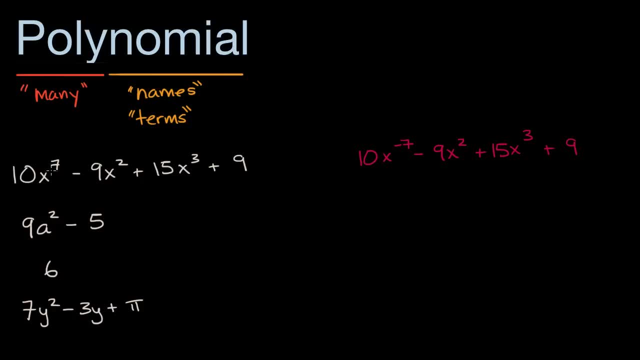 for what makes something a polynomial? that you have to have non-negative powers of your variable in each of the terms- And I just used that word terms- so let me explain it, because it'll help me explain what a polynomial is. A polynomial is something that is made up. 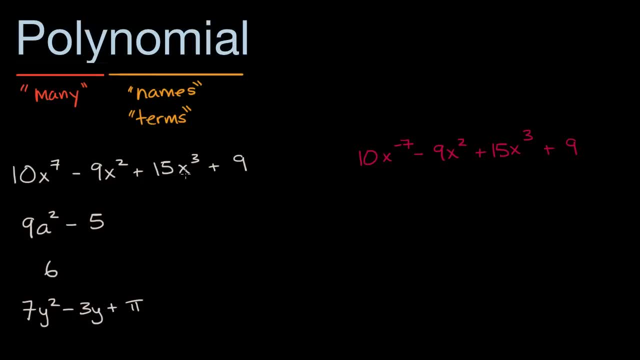 of a sum of terms, And so, for example, in this first polynomial, the first term is 10x to the 7th. The second term is negative 9x squared. The next term is 15x to the 3rd. 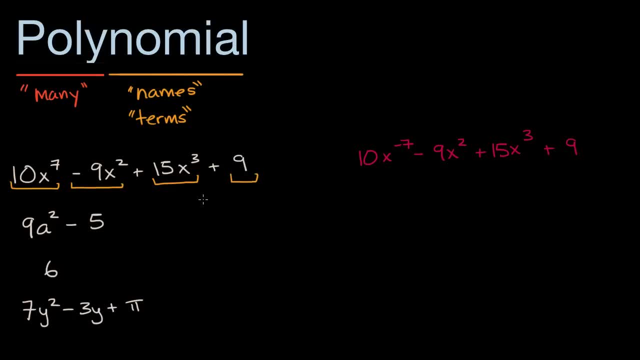 And then the last term. maybe you could say: the fourth term is nine And you can see something. let me underline these. So these are all terms. This is a four-term polynomial. right over here And you could say: hey, wait. 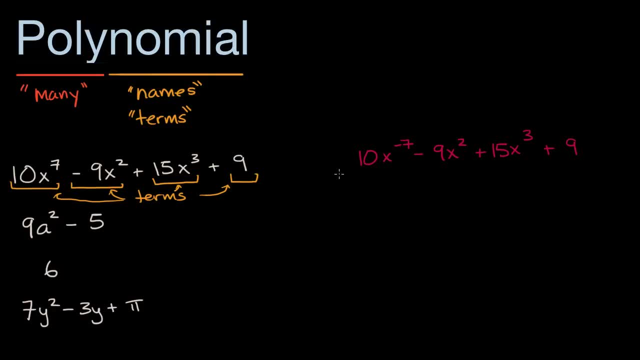 this thing you wrote in red. this also has four terms, But we have to put a few more rules to officially be a polynomial, especially a polynomial in one variable. Each of those terms are going to be made up of a coefficient. This is the thing that multiplies the variable to some power. 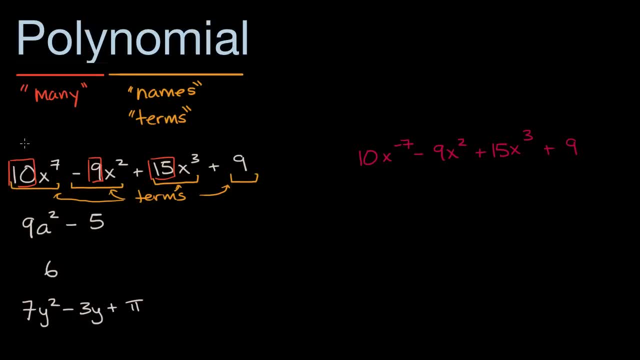 So in this first term, the coefficient is 10.. And let me write this word down: coefficient. It's another fancy word, but it's just a thing that's multiplied, in this case times the variable, which is x to the 7th power. 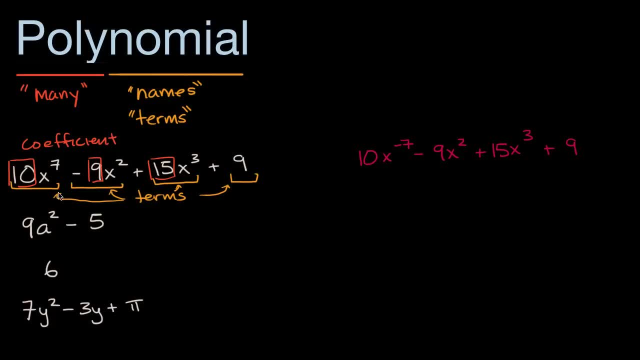 So the first coefficient is 10.. The next coefficient- and actually let me be careful here, because the second coefficient here is negative- nine. So we are looking at coefficients. The third coefficient here is 15.. And you can view this fourth term. 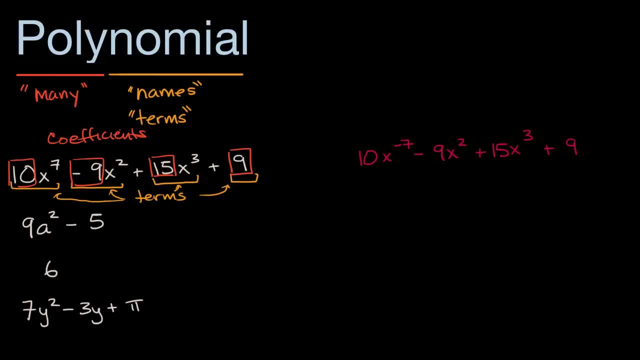 or this fourth number as the coefficient, because this could be rewritten as: instead of just writing it as nine, you could write it as nine, x to the zero power, And then it looks a little bit clearer like a coefficient. So in general, a polynomial is the sum. 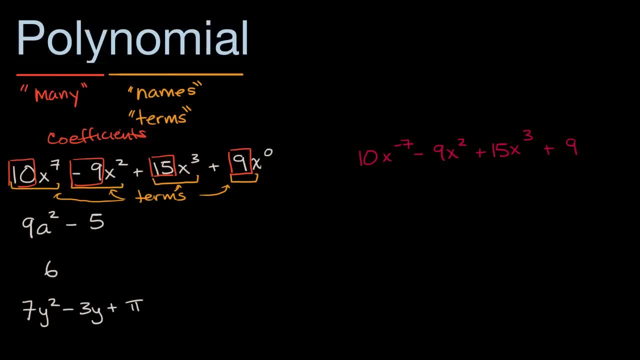 of a finite number of terms where each term has a coefficient which I could represent with the letter a being multiplied by a variable, being raised to a non-negative integer power. So this right over here is a coefficient. It can be if we're dealing 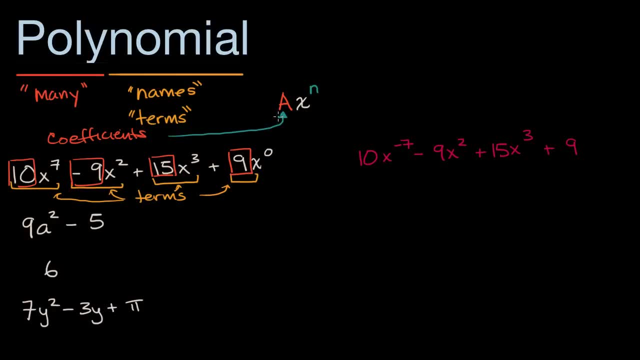 well, I don't want to get too technical. we could give a positive, negative number, It could be any real number. We have our variable And then the exponent here has to be non-negative, Non-negative integer. So here the reason why what I wrote in red: 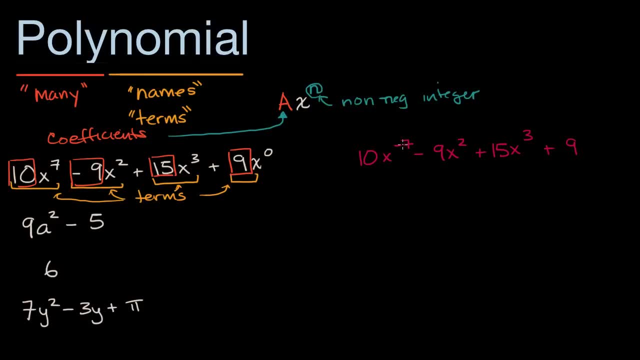 is not a polynomial is because here I have an exponent that is a negative integer. Let's give some other examples of things that are not polynomials. So if I were to change the second one to, instead of nine a squared, if I wrote it as nine a to the 1 1⁄2 power minus five, 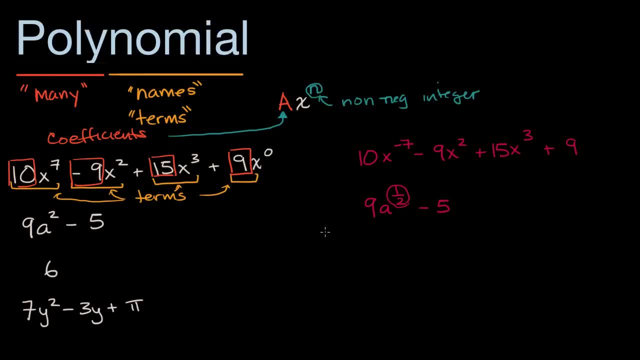 this is not a polynomial, because this exponent right over here it is no longer an integer, it's 1 1⁄2.. And this is the same thing as nine times the square root of a minus five. This also would not be a polynomial. 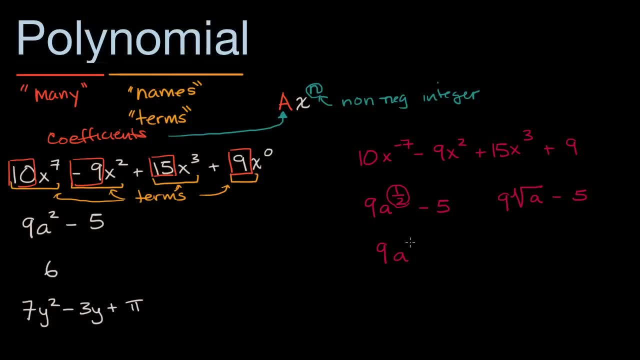 Or if I were to write nine a to the, a power minus five, also not a polynomial, because here the exponent is a variable, It's not a non-negative integer. So all of these are examples of polynomials. So there's a few more pieces of terminology. 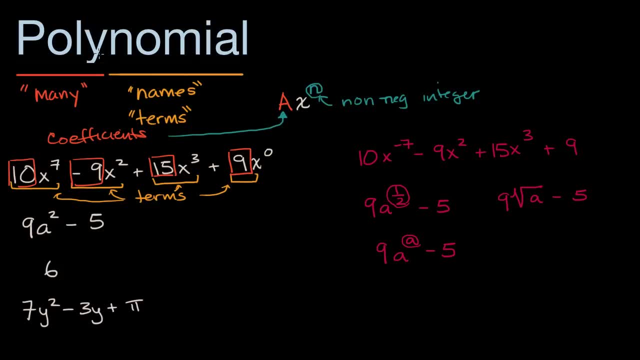 that are valuable to know. Polynomials is a or a. polynomial is a general term for one of these expressions that has multiple terms, a finite number, so not an infinite number, and each of the terms has this form, But there's more specific terms. 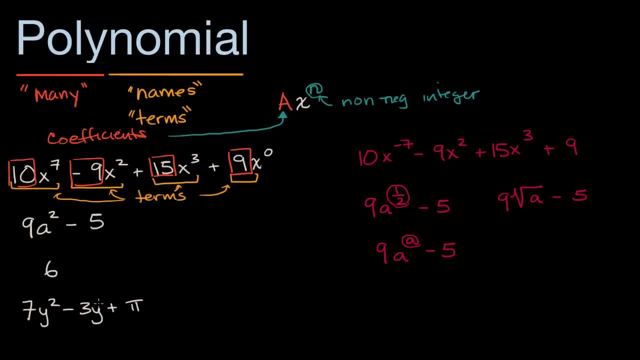 for when you have only one term or two terms or three terms. So when you have one term, it's called a monomial. So this is a monomial. This is an example of a monomial which we could write as six x to the zero. 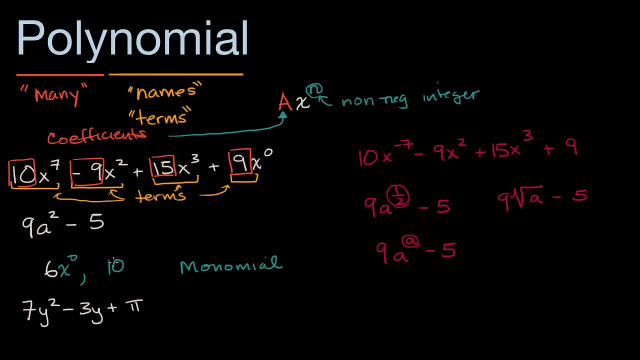 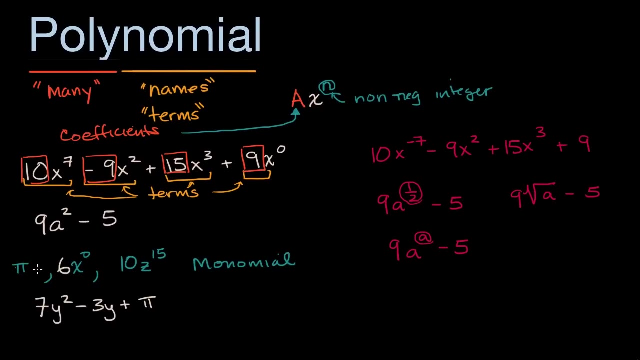 But you could also. another example of a monomial might be 10 z to the 15th power. That's also a monomial. Your coefficient could be pi, Pi, whoops, it could be pi, So we could write pi times times b to the fifth power. 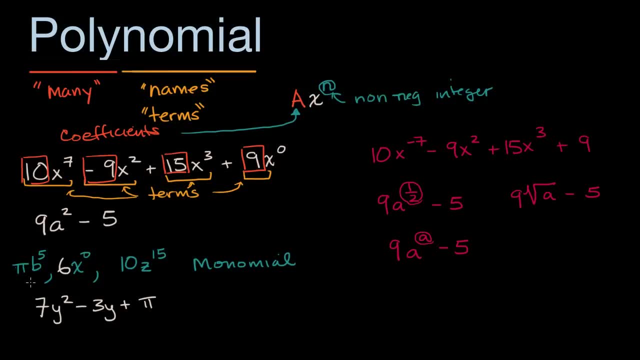 Any of these would be monomials. So what's a binomial? Well, a binomial is where you have two terms: Monomial, mono for one, one term. Binomial is you have two terms. So this right over here is a binomial. 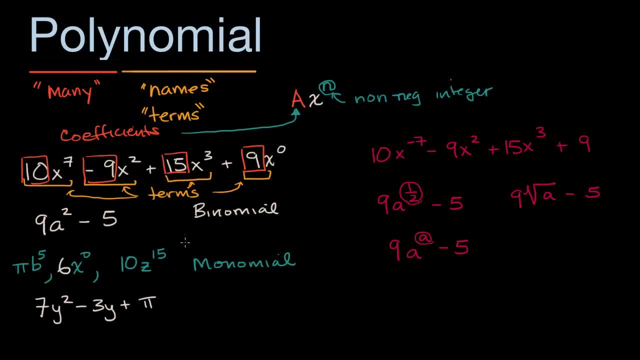 Binomial. You have two terms And all of these are polynomials, but these are subclassifications, So it's a binomial. you have one, two terms. Another example of a binomial would be: would be three y to the third plus five y. 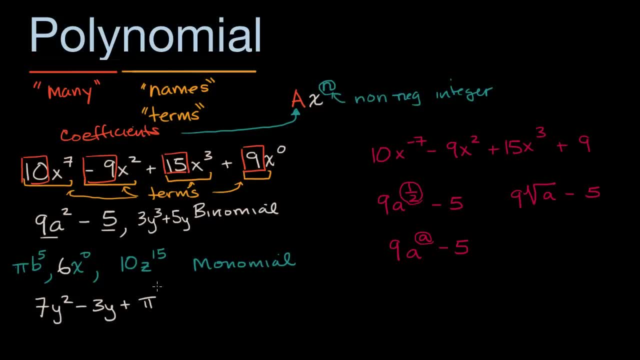 Once again, you have two terms that have this form. right over here Now you'll also hear the term trinomial. Well, trinomial is when you have three terms Trinomial, And this right over here is an example. 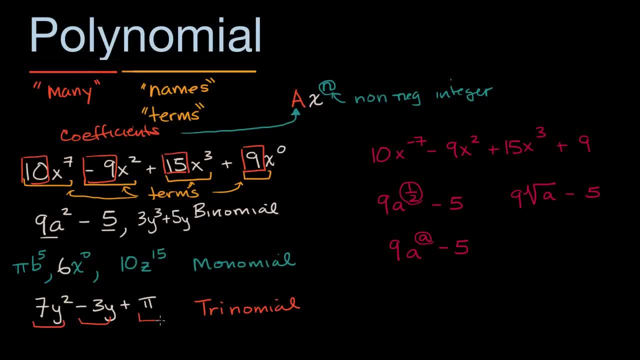 This is the first term, This is the second term And this is the third term. Now, the next word that you will hear often in the context with polynomials is the notion of the degree of a polynomial, And you might hear people say: 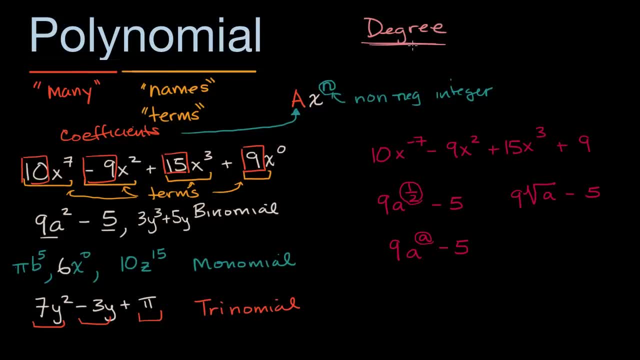 what is the degree of a polynomial, Or what is the degree of a given term of a polynomial? So let's start with the degree of a given term, So let's go to this polynomial. over here We have this first term, 10x to the seventh. 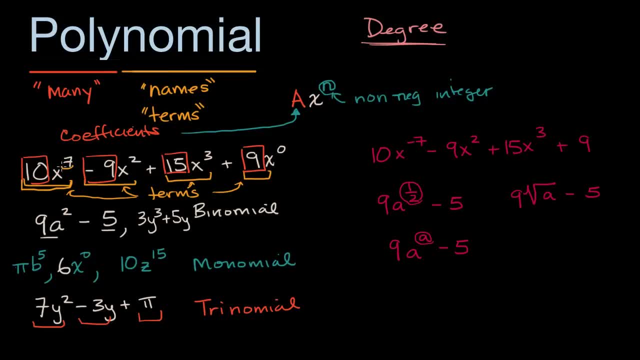 The degree is the power that we're raising the variable to. So this is a seventh degree term, The second term is a second degree term, The third term is a third degree term And you could view this constant term, which is really just nine. 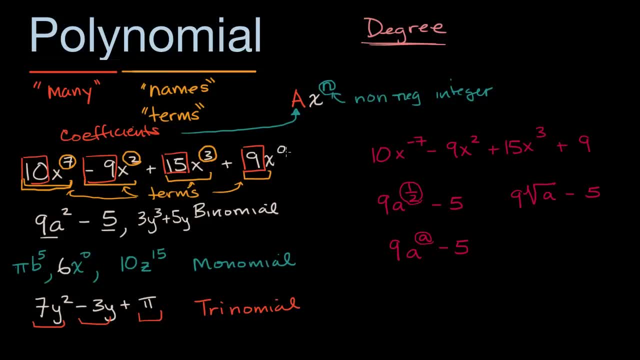 you could view that as sometimes people will say the constant term, sometimes people will say the zeroth degree term. Now, if people are talking about the degree of the entire polynomial, they're gonna say, well, what is the degree of the highest term? 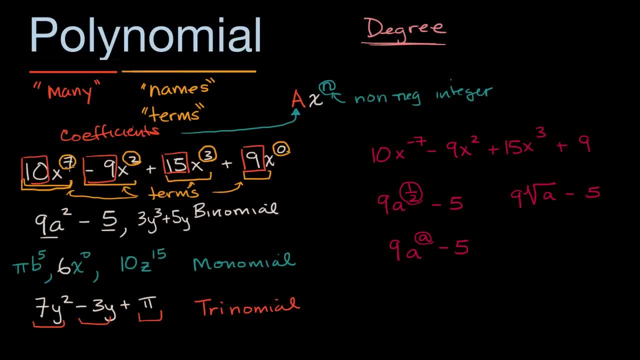 What is the term with the highest degree? That degree will be the degree of the entire polynomial. So this first polynomial, this is a seventh degree polynomial. This one right over here is a second degree polynomial because it has a second degree term. 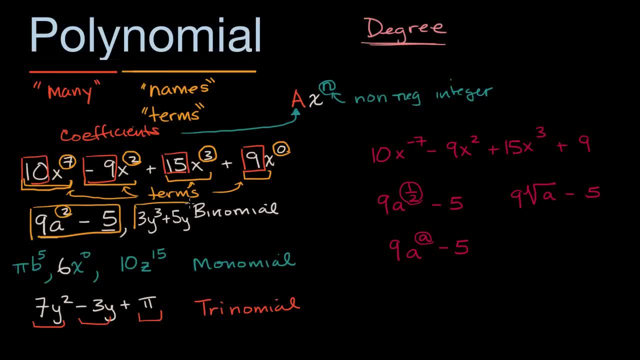 and that's the highest degree term. This right over here is a third degree. You could even say third degree binomial, because its highest degree term has degree three. If this said five y to the seventh instead of five y, well then it would be a seventh degree binomial. 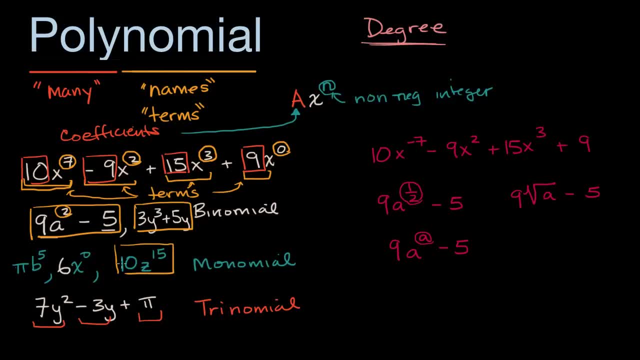 This right over here is a 15th degree, and this is a 15th degree monomial. This is a second degree, trinomial. Now, the last thing I will, or a few more things I will introduce you to, is the idea of a leading term and a leading coefficient. 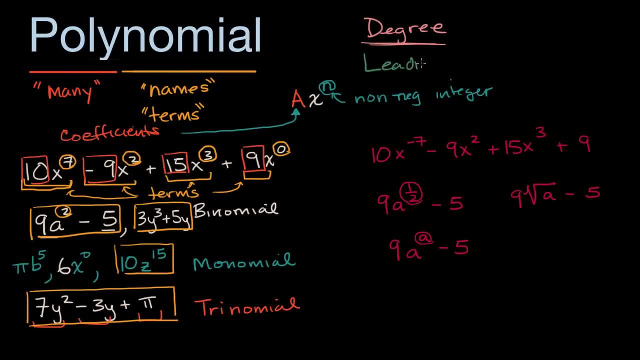 So let me write this down: the notion of what it means to be leading. Well, it usually means, it can mean whatever is the first term or the coefficient. If you're saying leading term and if you're saying leading coefficient, it's the coefficient in the first term.